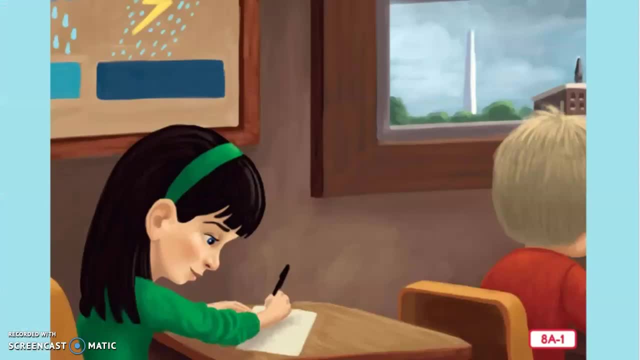 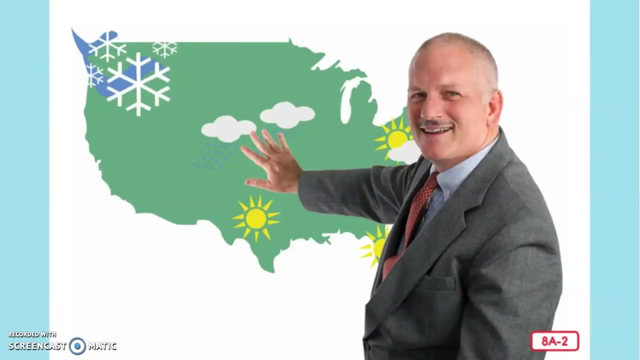 Dear kindergartners, this is my last letter to you about seasons and weather. Today, we will learn how to know what kind of weather is on the way. Have you ever watched the weatherman or weatherwoman on the news? Sometimes people blame the weatherman for bad weather especially. 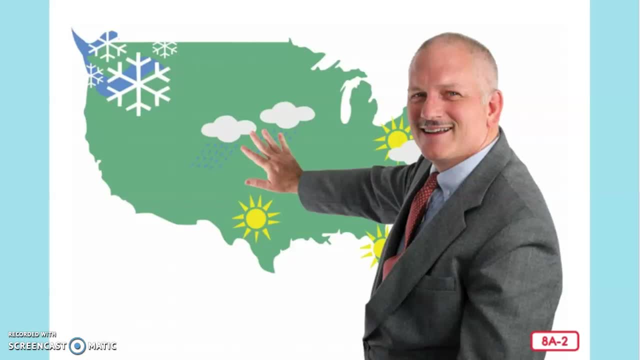 when their plans are spoiled. If you have a weatherman or weatherwoman on the news, have you ever watched the weatherman or weatherwoman on the news? Sometimes people blame the weatherman for bad weather. nada, How did you know? he was not being spoiled by the rain, But the 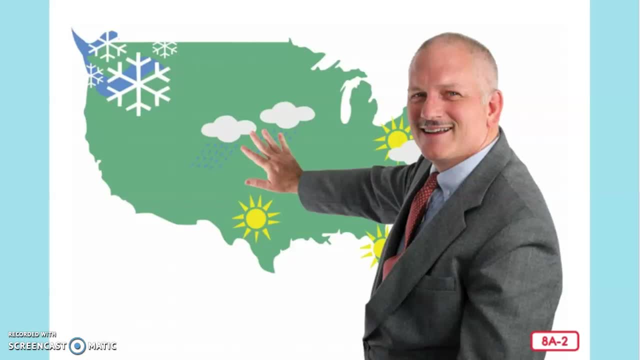 weatherman does not control the weather. He just tries to predict or make his own best guess at what the weather is going to be like later in the day, tomorrow or next week. Sometimes he is right and sometimes he is wrong. The study of weather and making weather predictions is called meteorology, and the person who 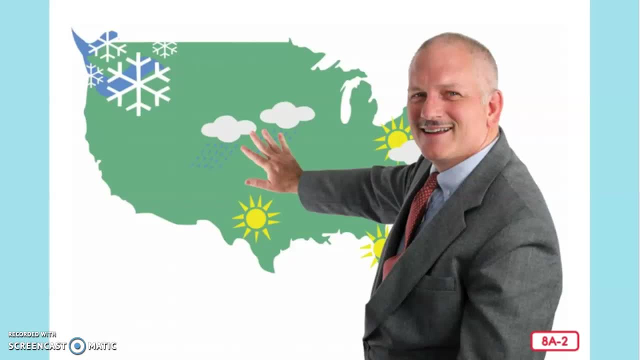 does. this is called a meteorologist. The words weatherman and weatherwoman are sometimes used to describe weather events. or That's right, weather is sleepwalking people who appear on television to tell you about the weather. Maybe you've seen them on the news. Often, weatherman or weatherwoman is a meteorologist. 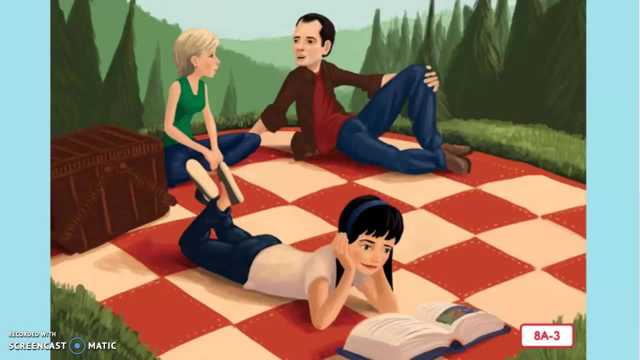 Oops, sorry, forgot to take a picture. Predicting weather is more important, so people will know what to wear that day and whether or not they need an umbrella because of the rain. Predicting weather also helps people to plan things like picnics or. 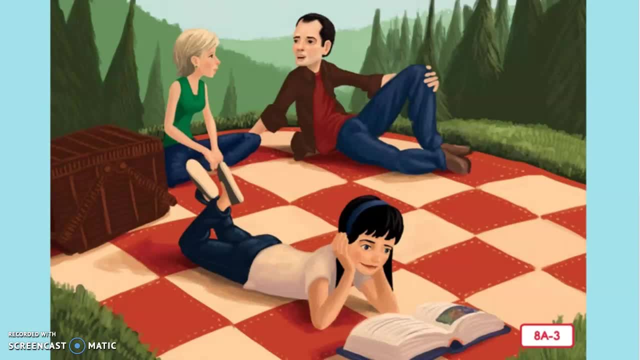 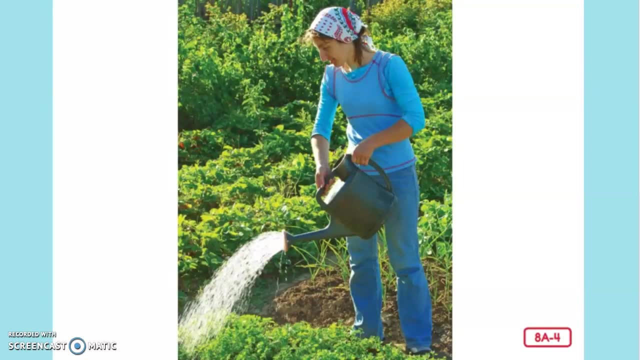 trips to the beach. If my parents are planning a family picnic, for example, they would want to make sure that it's not going to rain on us while we are outside. but picnickers and vacationers are not the only ones who care what meteorologists. 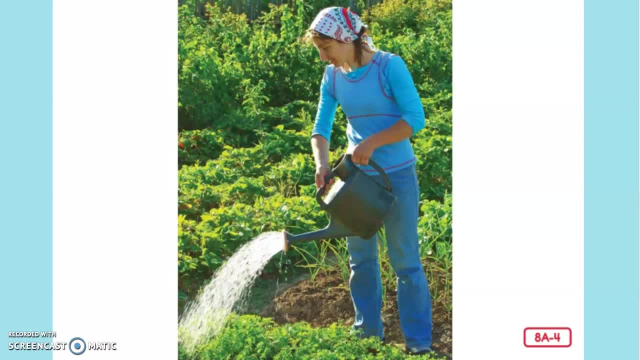 have to say. Farmers need to know how much rain to expect. If the meteorologist says it's not going to rain for a while, PEARLS Farmers may need to figure out another way to get water to their plants. In fact, anyone whose job can be affected by the weather needs a meteorologist. 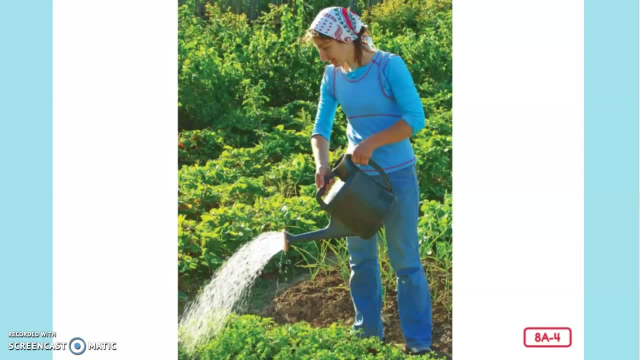 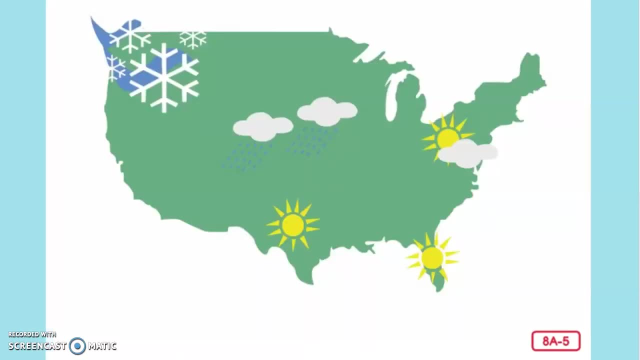 whether the person is a baseball player, a construction worker or a garbage man, or an airline pilot or an astronaut. One way meteorologists predict what the weather will be like in the future is by studying weather patterns and temperature from the past. 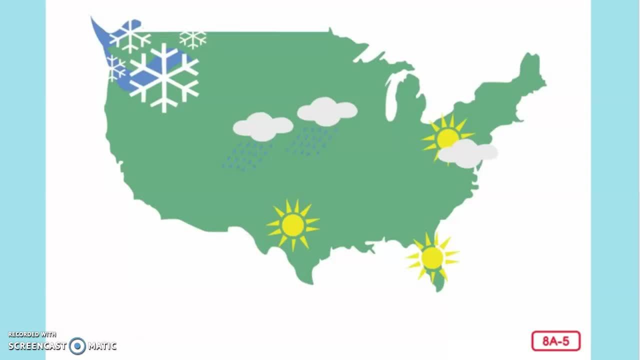 When you watch a weather report, the weather person will tell you what the high or warmest temperature and the low or coldest temperature will be for the day. High temperatures usually come during the daytime and low temperatures are usually at night. However, the weather person can also tell you if the temperatures on a particular day are normal for that time of year by checking the weather record. 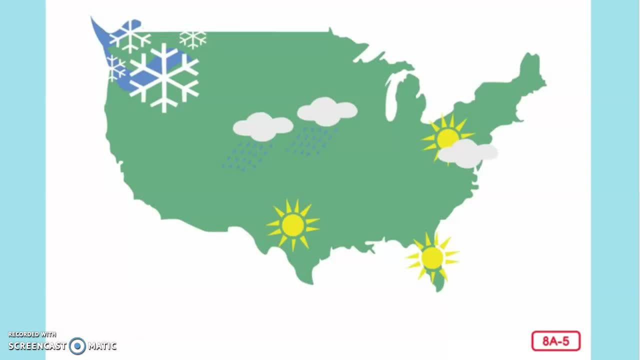 The weather record is kind of like a weather diary. It lists the weather and what it was like on that day in previous years. Aside from looking at weather records, what else do meteorologists use to predict the weather? How do you know what is going to happen? 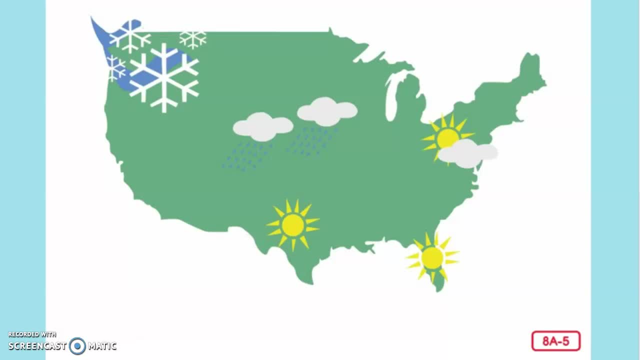 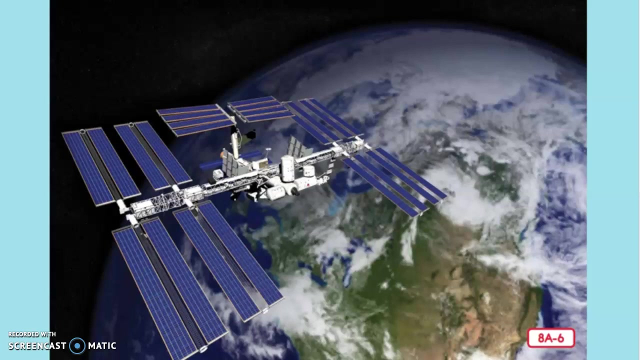 In fact, predicting the weather is quite complicated, And even with all the amazing computers and equipment we have nowadays, the weather person is still sometimes wrong. Meteorologists' predictions are also correct a lot of the time too. This is thanks in part to satellites like the one in this picture. 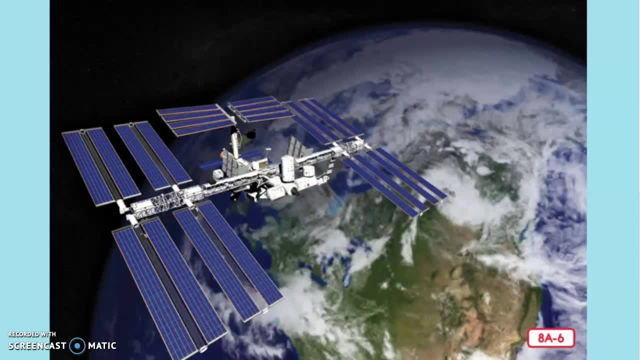 Satellites are objects launched into space that contain cameras, radios, antennas, but no people. Once in space, the satellites travel all around the world. The satellite cameras take pictures and beam them down to the meteorologist. Using photos, meteorologists can see storms and storms. 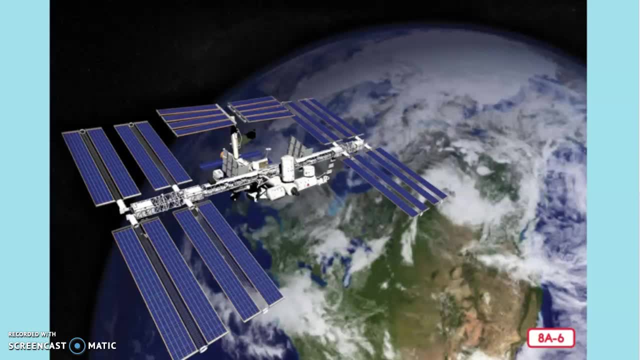 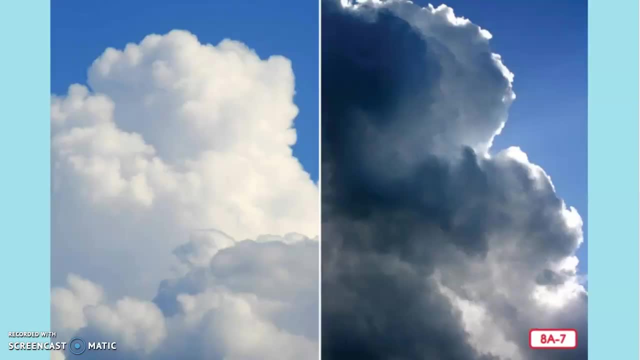 Using photos, meteorologists can see storms and storms As they develop and predict weather. the skies will be clear or cloudy. Of course, you don't always need a meteorologist to tell you the weather and what it's going to be like. 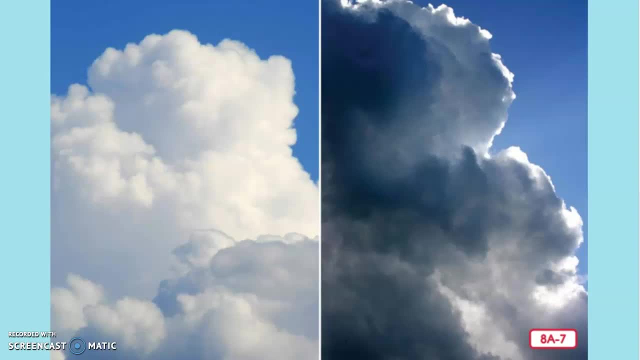 especially if dark clouds like this roll over your town. These dark clouds are types of cumulus clouds and often develop into thunderstorms. You can also find cumulus clouds during nice weather, when they appear white and puffy like a cotton ball. You can also find cumulus clouds during nice weather, when they appear white and puffy like a cotton ball. 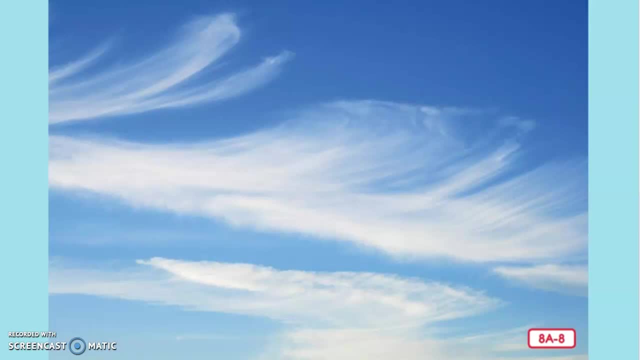 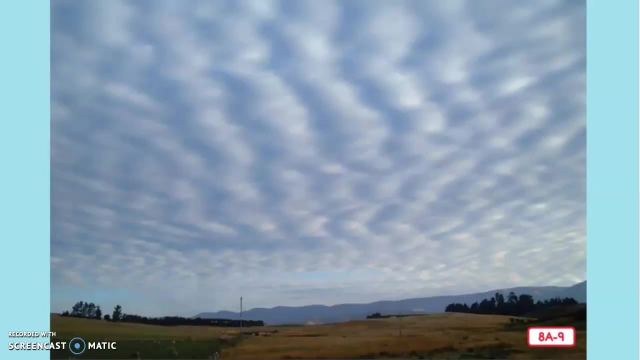 These are cirrus clouds. They are thin and wispy clouds that float way up in the sky. Usually, cirrus clouds mean the weather is going to be clear and pleasant. They are usually thin and wispy. Stratus clouds are the third cloud type and they float fairly low to the ground. 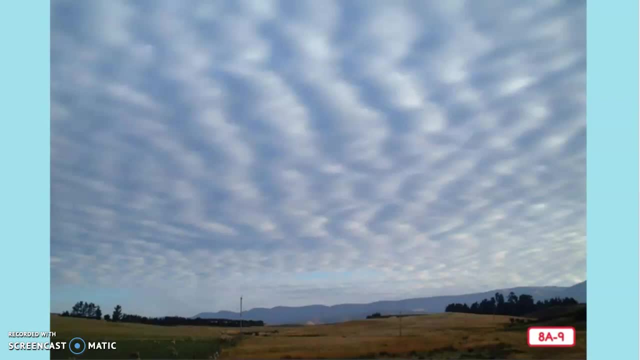 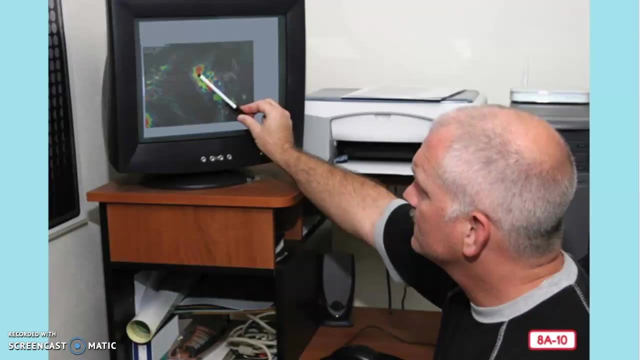 These flat clouds can stretch across the entire sky. These clouds can stretch across the entire sky. They sometimes reach up to the ground. These flat clouds can stretch across the entire sky. They sometimes reach up to the ground from light, rain or drizzle. The most important part of a meteorologist's job is to help save. 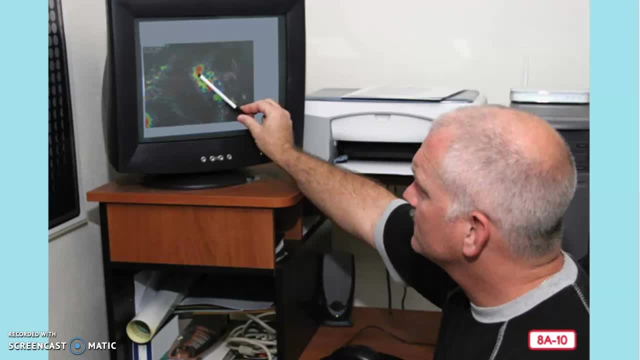 lives by warning people when severe weather is on the way. Look at this picture. It was taken when a hurricane was heading toward land. A hurricane is a huge storm that forms out over the ocean. The meteorologist in this picture is studying images of a hurricane- just as it is about. 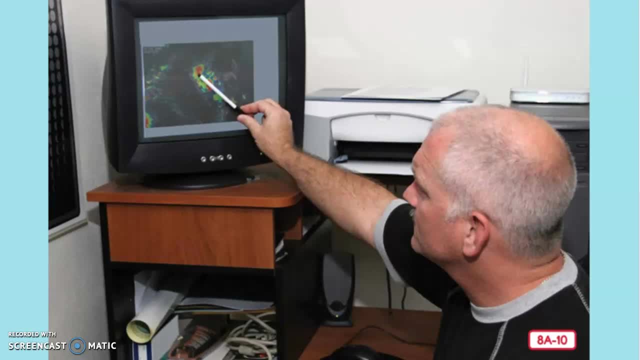 to strike land. The image was made by a computer that is able, thanks to satellites, airplanes and other tools, to determine how fast the wind is moving, how much it is raining and in which direction the storm is moving. Thanks to computers and satellites, the meteorologist saw the hurricane. 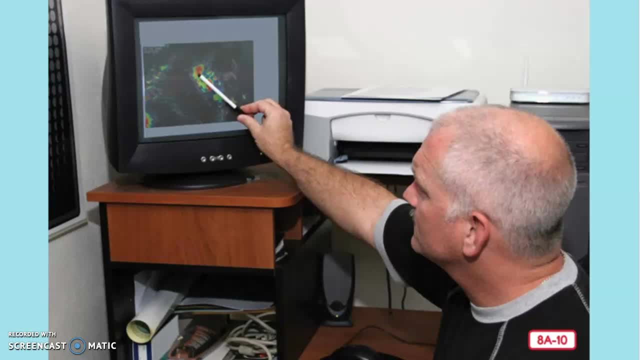 days before it came anywhere near land, so they warned the people to leave their homes and head to safer ground if necessary. A lot of people were kept safe, but the meteorologist was able to save a lot of people from this severe weather. Meteorologists help people stay prepared for and safe. 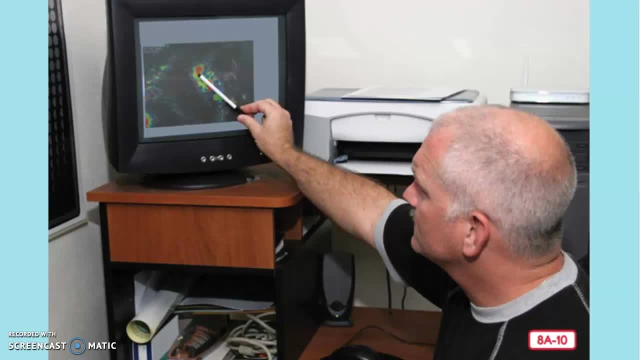 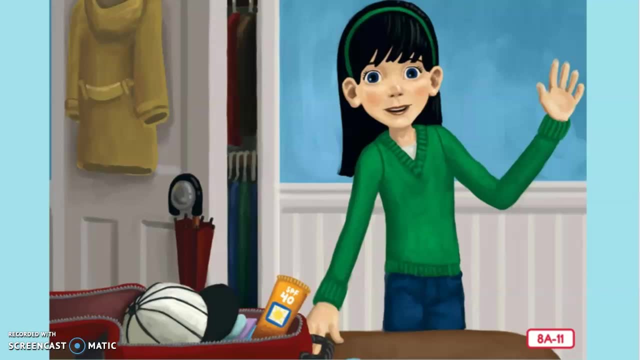 during storms and whatever challenges the weather may throw at you. Even though you can predict what the weather should be like during any given season where you live, it is difficult to always predict from day to day and exactly what the weather will really be like, so it's a good idea to listen to. 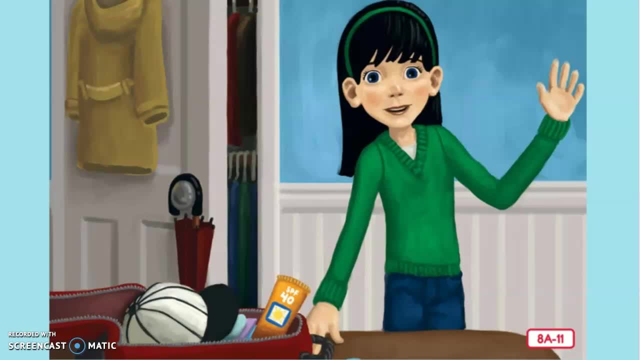 your local weatherman or weather woman so you look, so they can tell you to carry an umbrella on that day or to bring along some extra sunscreen. that way you'll always be prepared. thank you so much for helping me with my weather project. from now on, i hope you'll keep an eye to the sky and 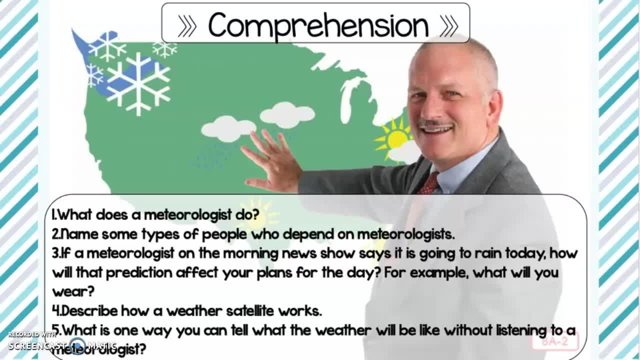 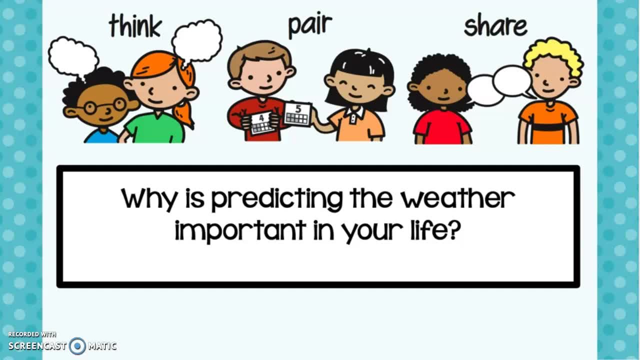 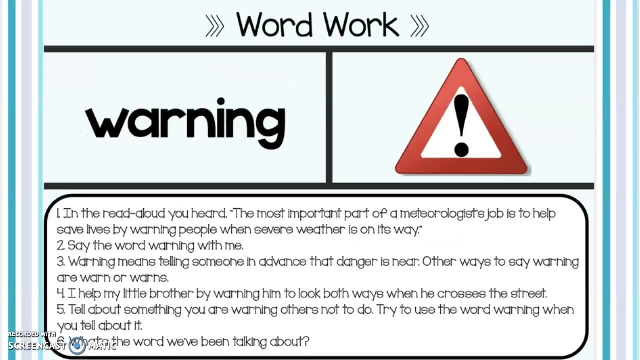 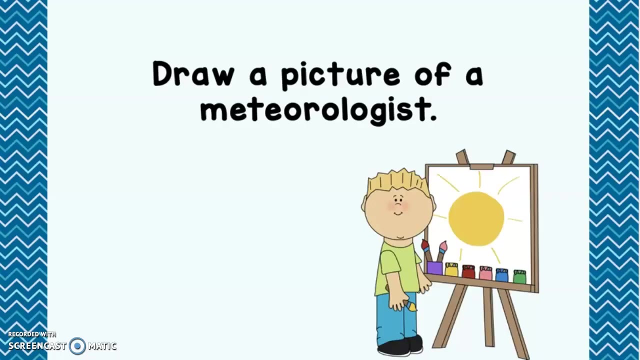 always: pause for discussion and play when you're ready. pause for discussion, play when you're ready. pause and play when you're ready. pause and play when you're ready. this is going to be where you can draw a picture of a meteorologist in your journal. this is a sentence you can write about the meteorologist.